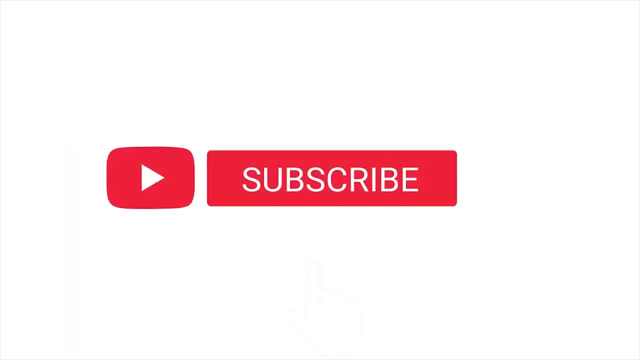 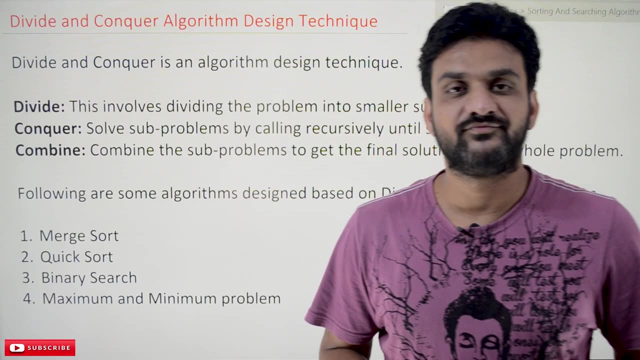 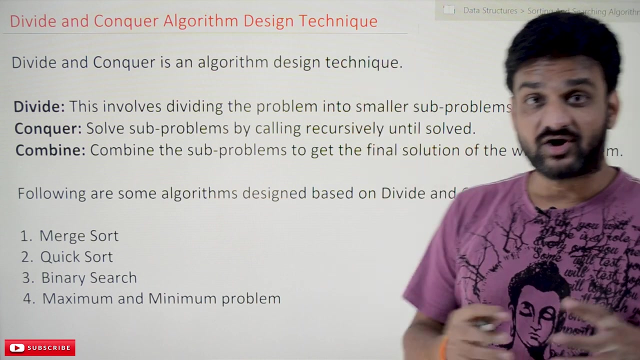 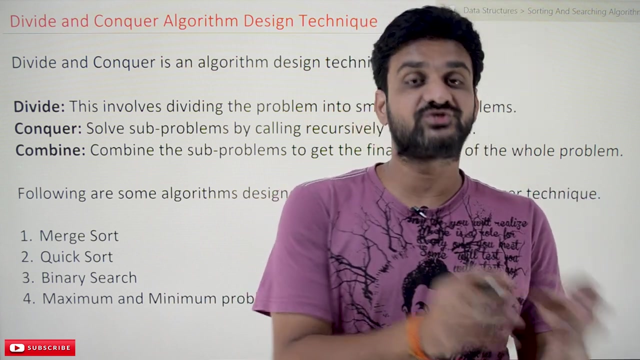 Hi, welcome to Learning Monkey. I am Vikram. In this class we will try to understand divide and conquer algorithm design technique, The concept of. in our previous classes we have discussed some of the sorting algorithms. If you haven't watched those videos, please watch those videos and come back here. 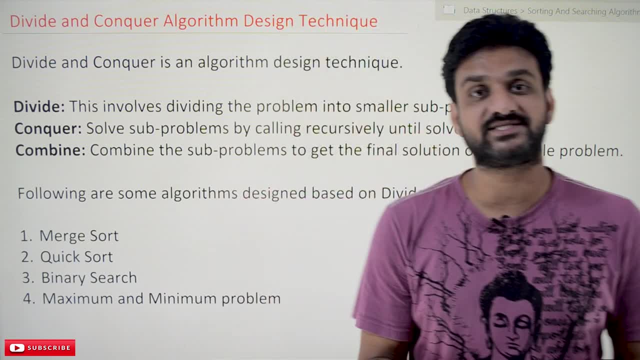 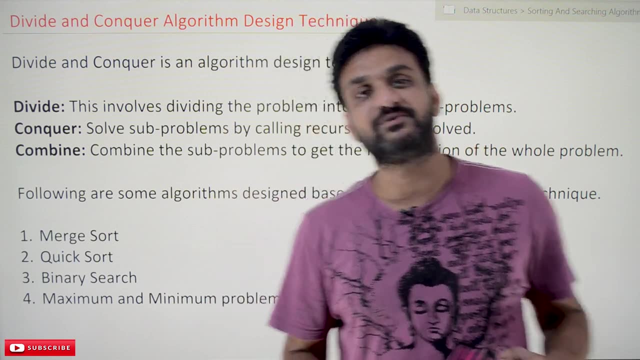 And every video in our channel is going to be a part of entire course or a playlist. Our suggestion is to follow the entire course so that you can have better understanding of the concepts. The link for the playlist is provided in the description below. Now, coming to this class, we will try to understand a design technique called divide and conquer. 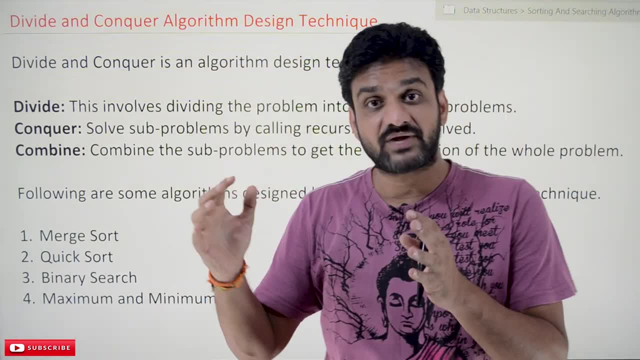 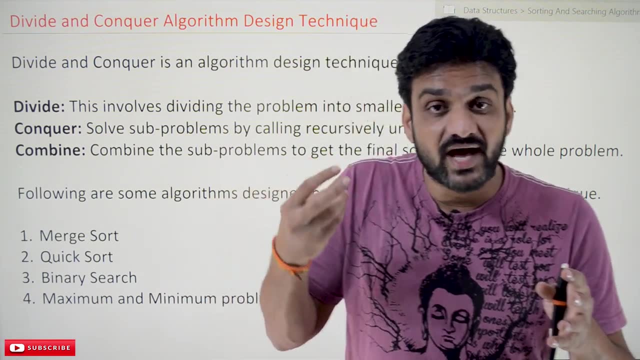 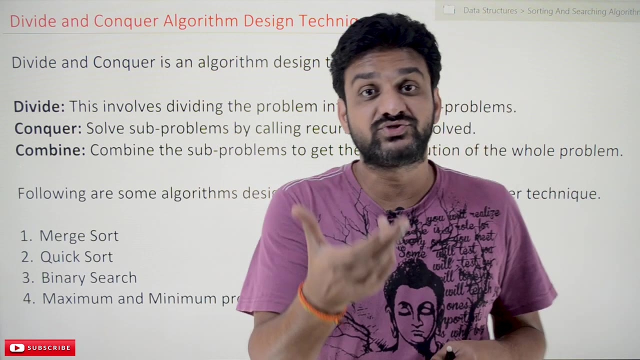 So there are some algorithms which are developed based upon this design technique called divide and conquer, And for this algorithm, in order to design the algorithms based upon this technique, we need to understand. So these design techniques are developed based by using. 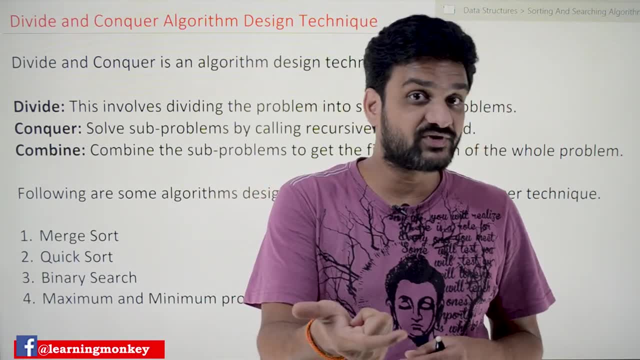 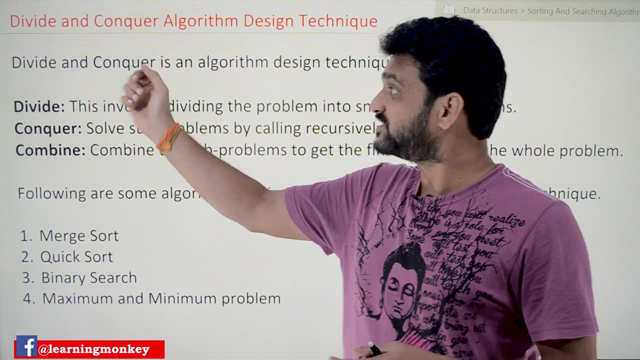 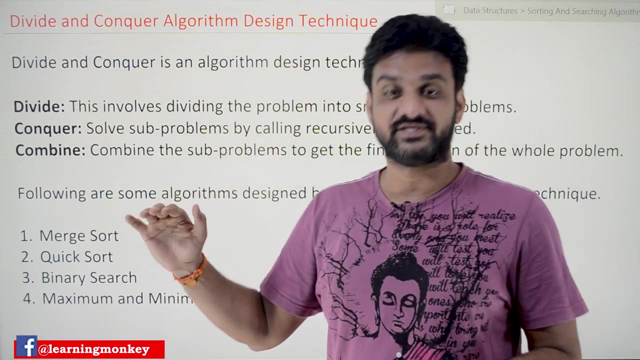 recursive algorithms. So the concept of recursion has already been explained. So, based upon those recursion concepts this divide and conquer is based, And what is this technique, and how this technique is going to solve the problems That we will try to understand. 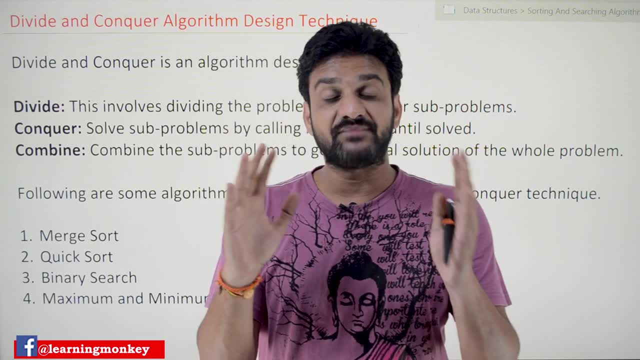 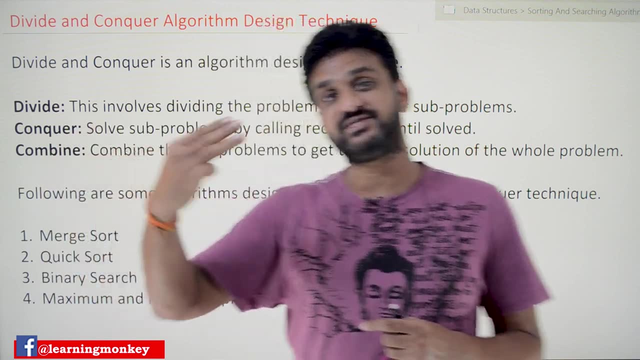 For example, if you have a problem, there are some problems which can be solved by using this technique called divide and conquer. So what is divide means? So there are three steps, The three steps that are going to be followed by divide and conquer. 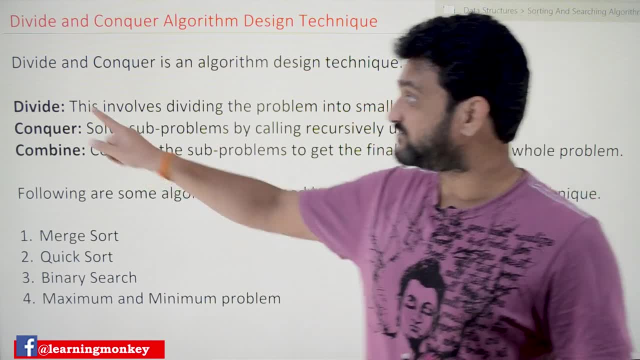 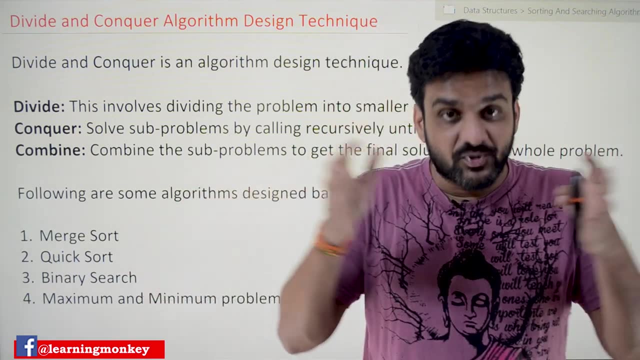 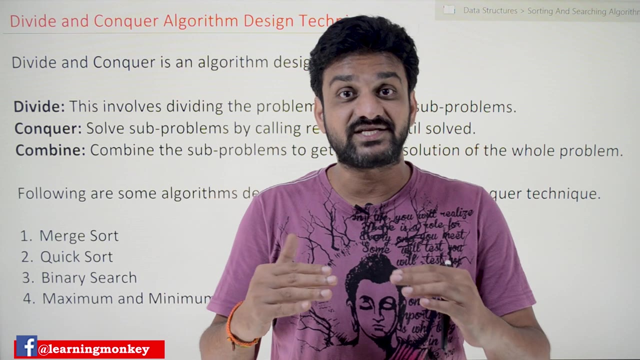 By this algorithm design technique, one is divide and the other one is conquer and the other one is combine. First, what it is going to do is, if you have a problem, that problem will be divided into sub-problems. So that problem will get divided into sub-problems to a certain extent, where that problem cannot be further divided. 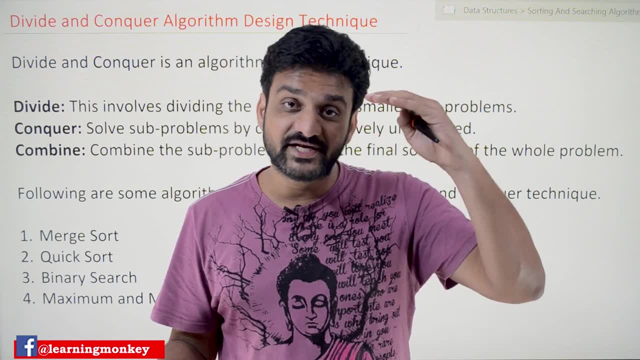 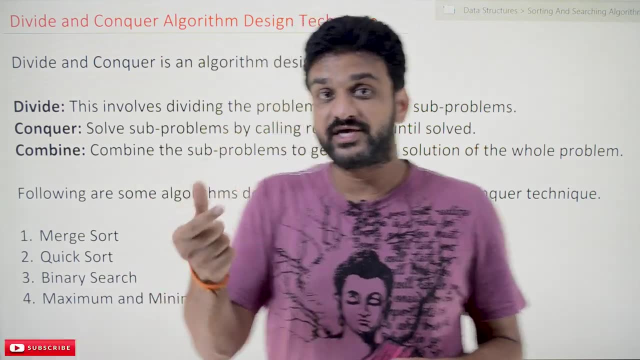 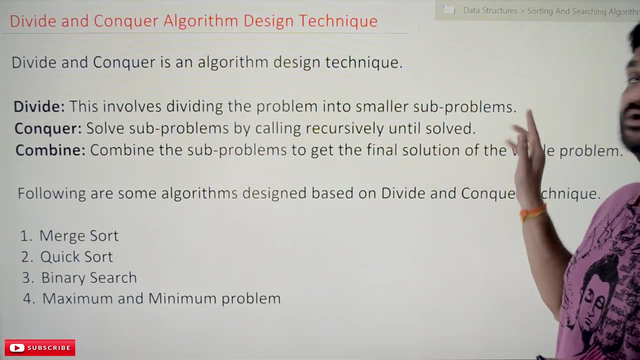 Okay So the small small pieces it is made. the entire big problem is made into small, small pieces, Small small problems. Okay. So the next step is conquer, Solve the sub-problem First is divide. This involves dividing the problem into smaller sub-problems. 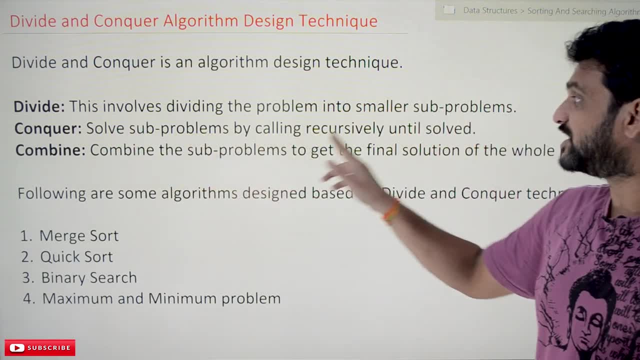 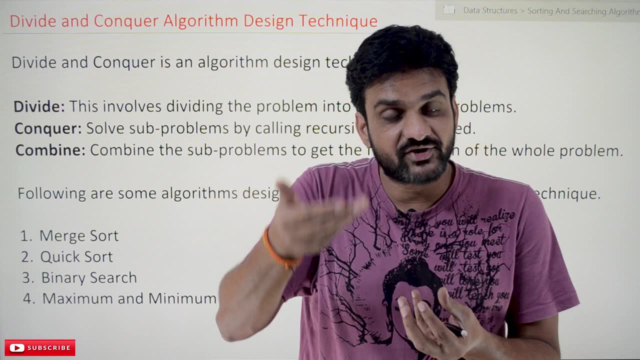 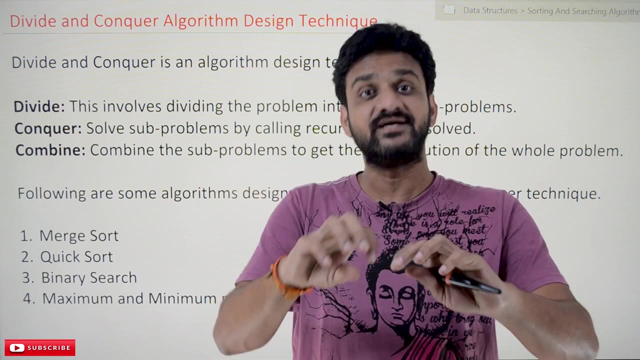 And the next one is conquer, Solve sub-problems by calling recursively until solved. So all those small, small problems are solved. So first we are going to divide and after dividing, so those small, small problems will get solved, All the small problems will get solved. 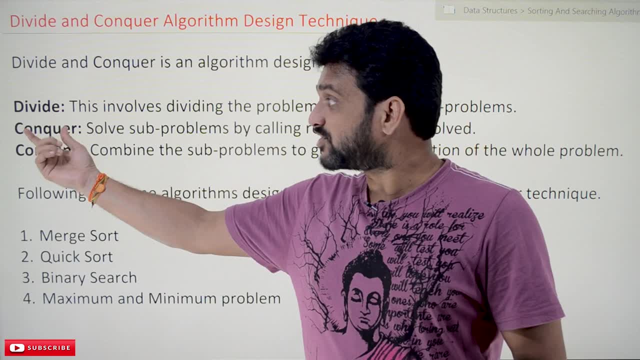 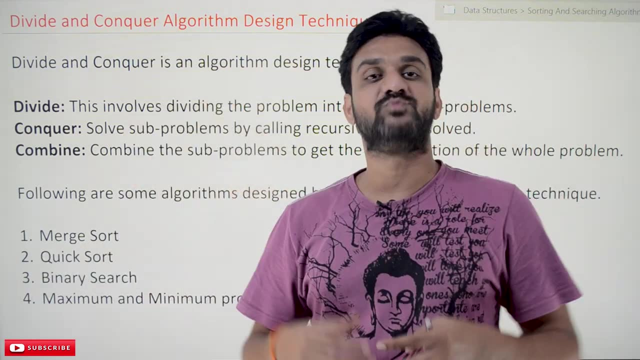 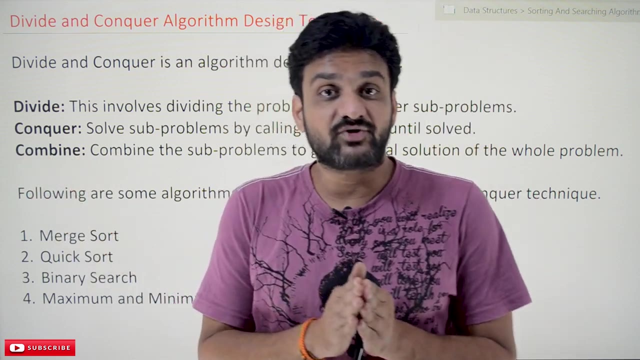 That is what we call it as conquer, That is the reason why we call this technique as divide and conquer. And the last step is combine. So, after solving the problems, again combine all those small, small pieces In the final attempt of combining. so in the final step of combining we are going to get the solution for the problem that we are having. 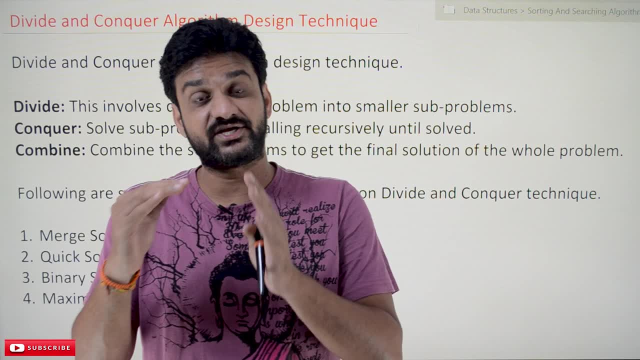 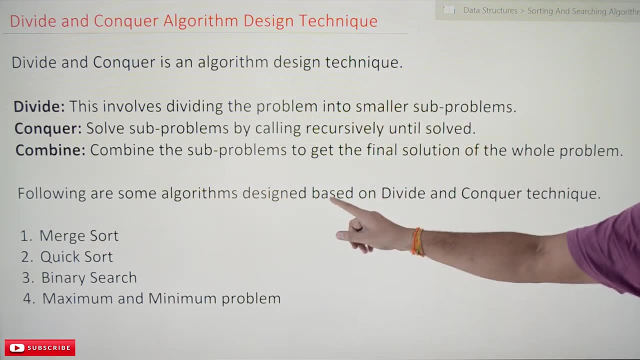 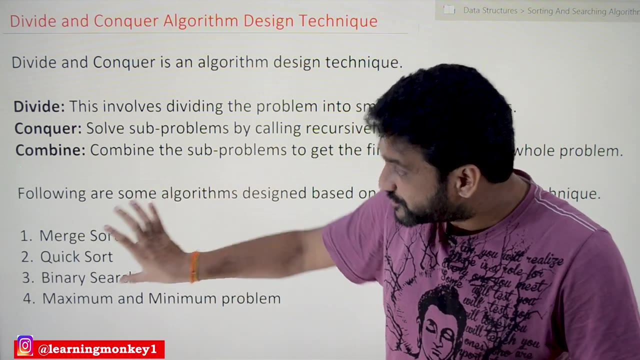 So how that is going to happen, we will try to understand. There are different algorithms which are designed based upon this divide and conquer. So the following are some of the algorithms designed based on divide and conquer technique. So these are the problems that are solved by using divide and conquer method. 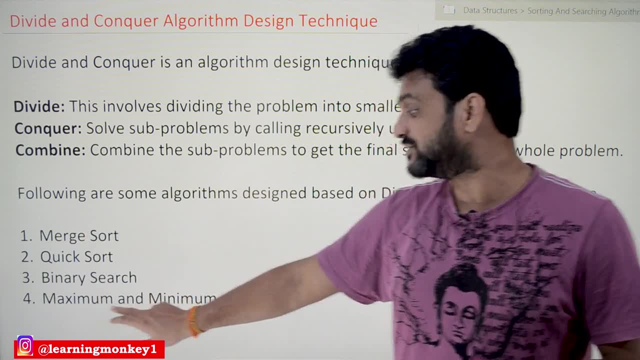 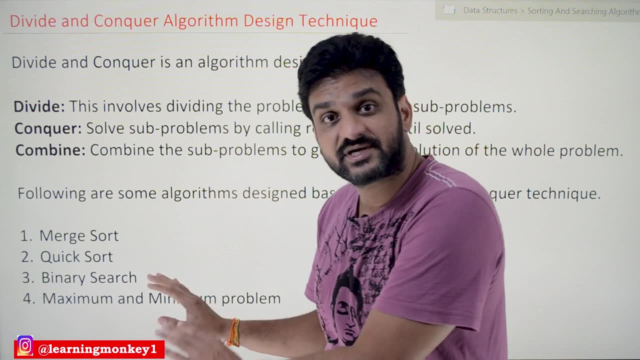 It is merge, sort, quick sort, binary search and min and max problem. So we are going to see each and every problem in detail in our later classes. So these problems are designed based upon the point that you have to understand is, these problems are based upon the concept of 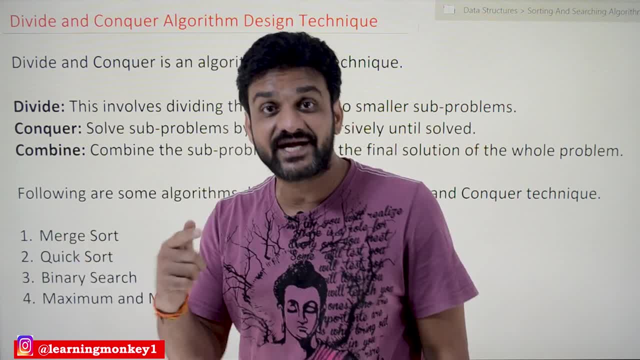 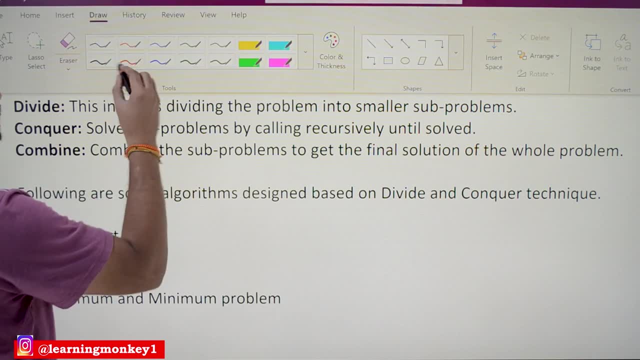 these problems are. the solutions for these problems are designed based upon the concept of divide and conquer. So, for better visualization, what we will do is so how this divide and conquer will work For that visualization. what we will do is so we will try to take a problem. 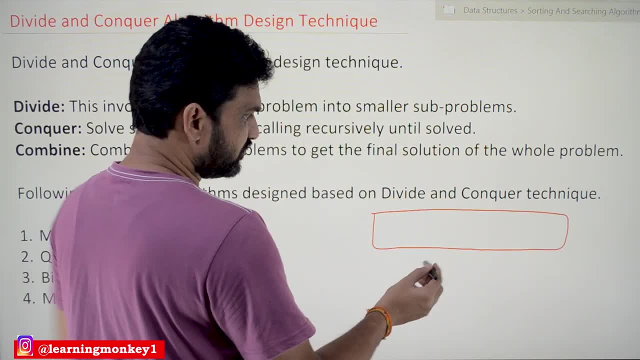 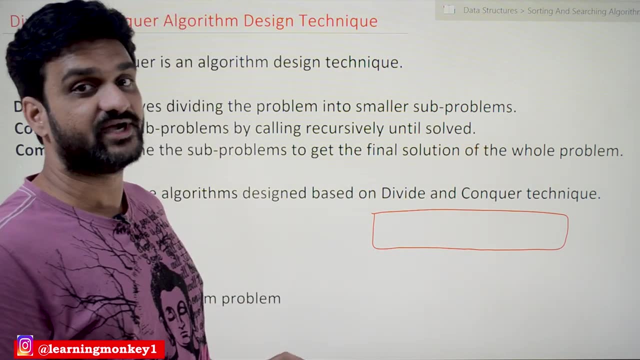 For example, assume that this is the problem, So, whatever it may be. So here we are having some problem and we are trying to find the solution for this problem by using divide and conquer How it works. How it works is: 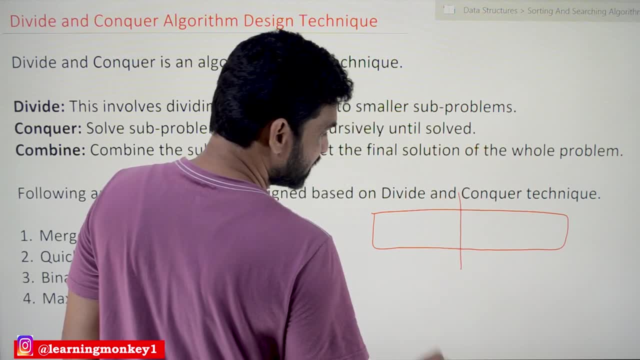 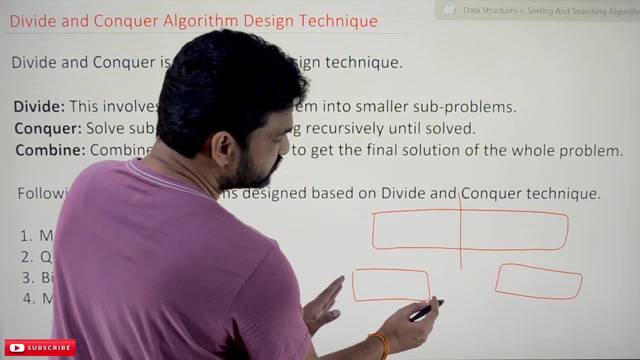 First, it is going to divide the problem. So it is going to divide the problem into small, small pieces It has made. so this entire problem is made into two pieces And again this problem will be made into another piece. another two pieces.